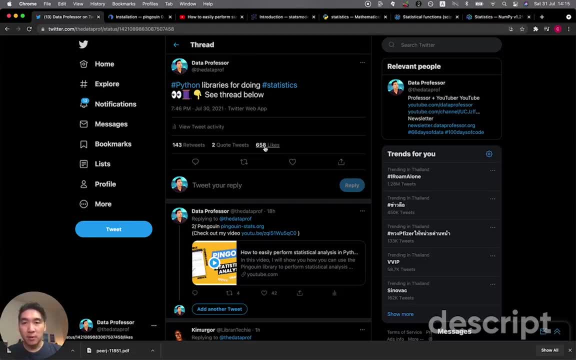 very quick video showing you some of the popular Python libraries that you could use for performing statistical analysis, And so, without further ado, we're starting right now. So the first library that I mentioned here is the penguin Python library, And I've actually made a quick video. 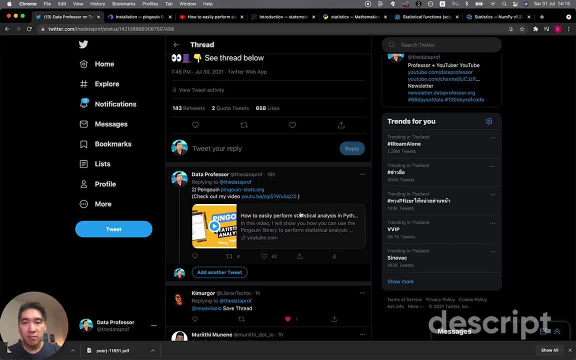 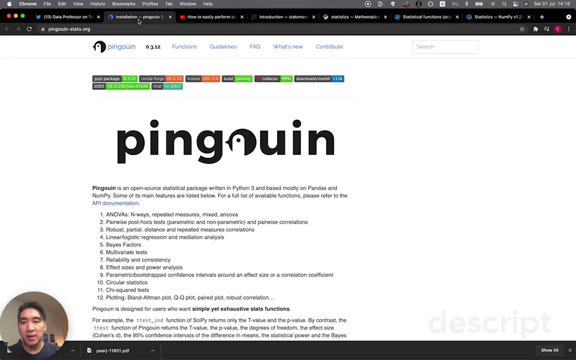 about that, showing you how to use this awesome library to perform several of the common statistical analysis in Python, And so you could definitely check this video out, And I'll provide you the links in the video description. And so let's head over to the penguins website here. 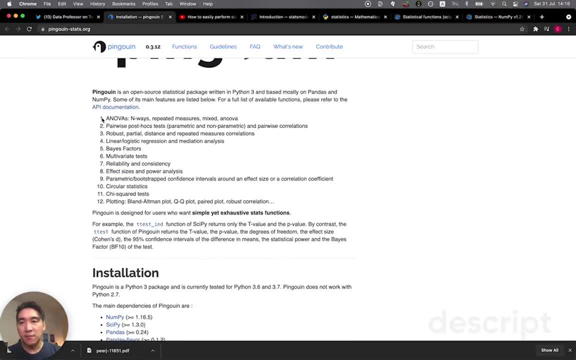 And so this is the front page, And here you can see that it provides a wide range of functionalities for you to perform. So some of the common statistical analysis, such as ANOVA, t-test, Bayesian stats, chi-square tests, etc. Even plots could also be created here in penguin, And so here are some example code that: 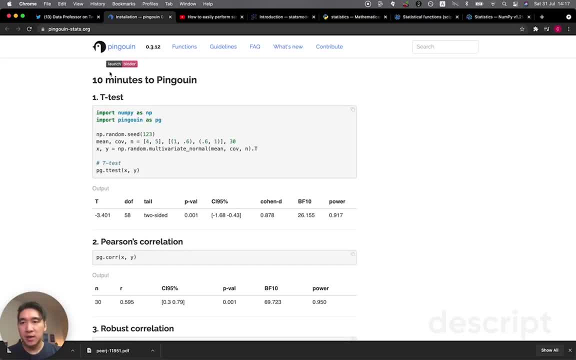 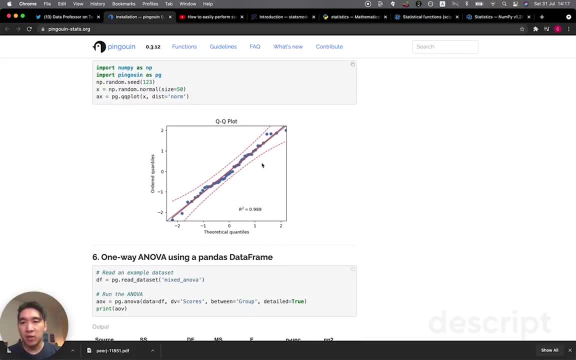 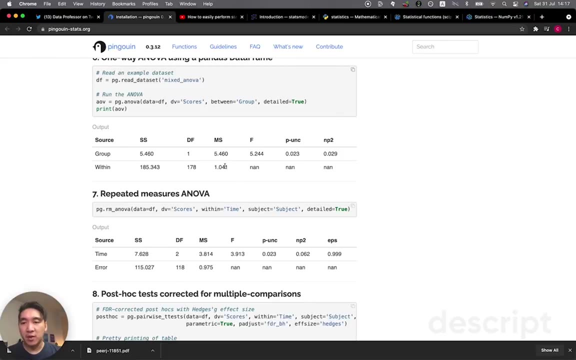 you could use for performing some t-test, And so you could follow along here for a 10 minute guide on how you could get started. All right, and it also comes pre equipped with this qq plot that you could test for the normality of your data sets. This is for ANOVA. 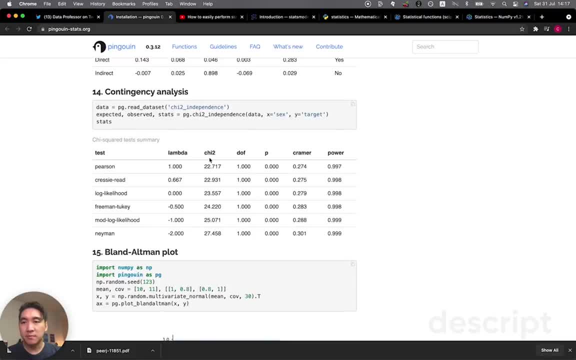 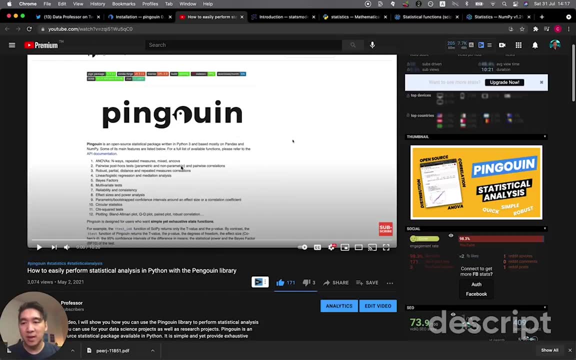 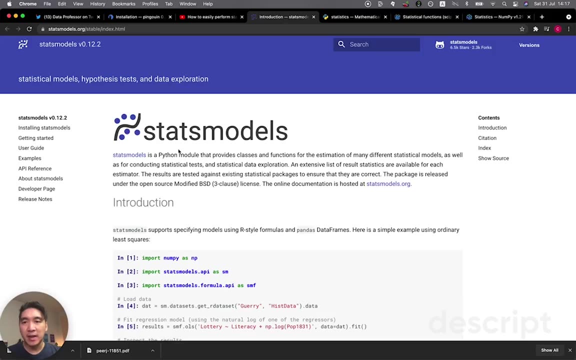 And you could also build some simple linear regression here as well. All right, and so do check out this Python library And also check out this video that I made quite some time ago, in May of 2021.. And so the second library that I talked about is the stats models, And the great thing, 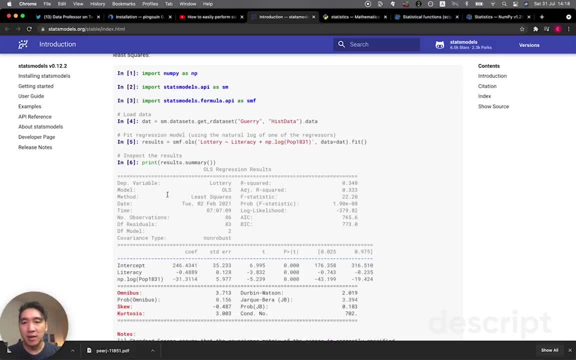 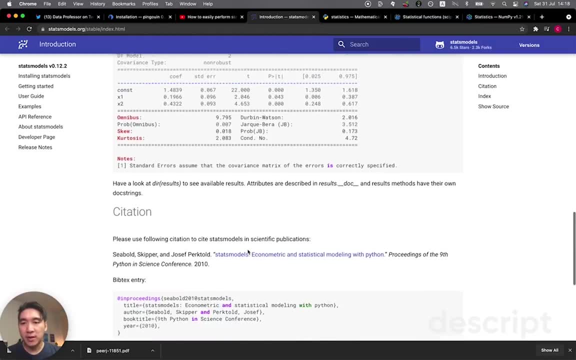 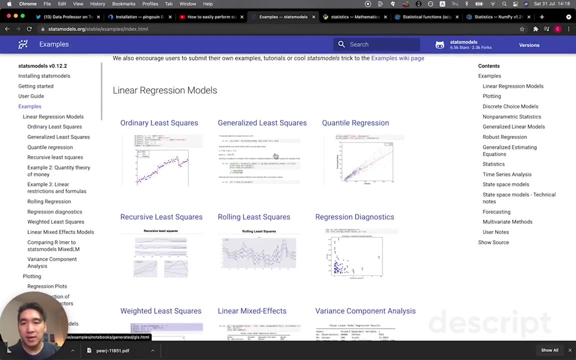 about the stats model is that it provides a very in depth analysis of the various statistical parameters of your model. And let's have a look further So you can see that they're pretty detailed. And let's check out the examples here So they provide you some example code for you to. 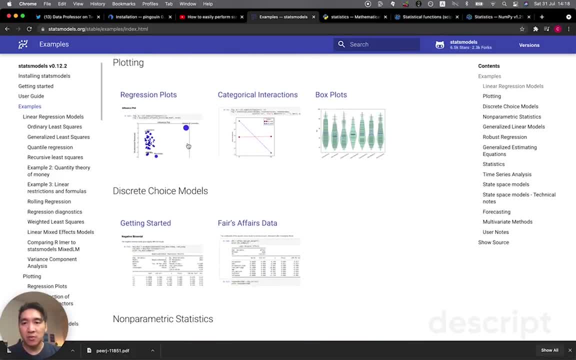 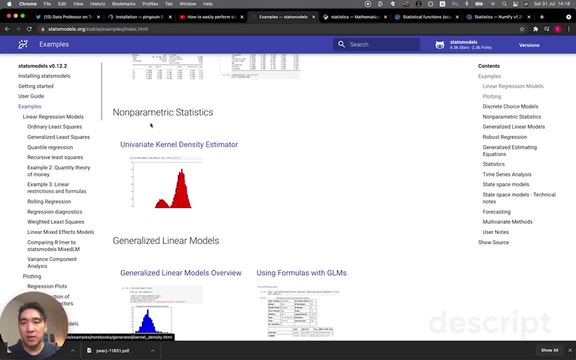 get started And they're conveniently grouped according to functionalities, Like, for example: here: you can make some regression plots, box plot or even do some non parametric analysis as well. So you can see here that there are quite a few functionalities. 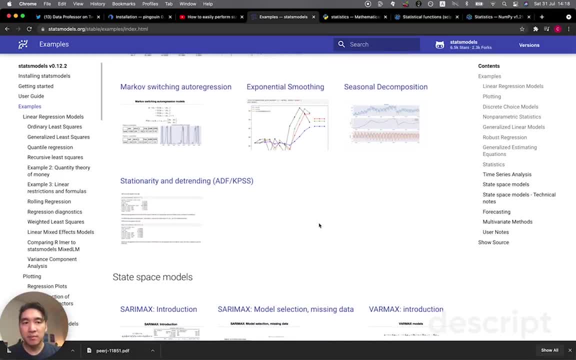 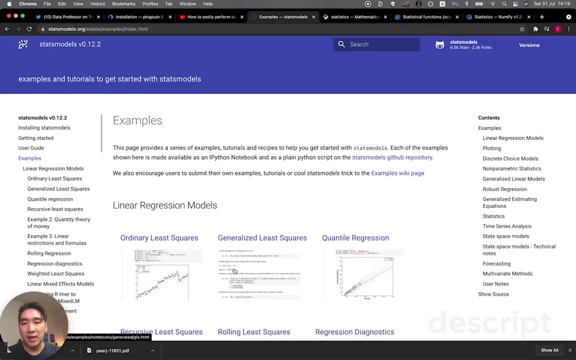 that you could perform here in the stats models, And so personally I use this model for performing some basic linear regression, and I really liked the statistical output that came out of it, And so you could check out this library, and I provide you the link as well in the video description. 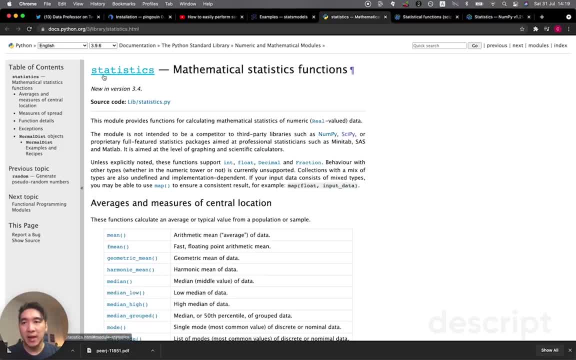 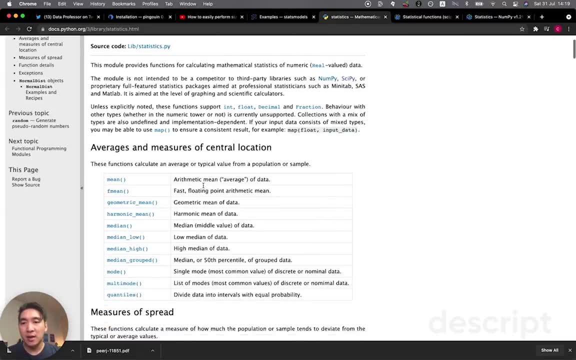 And let's hop on to the next one. So this one is quite basic and it comes pre equipped with the standard library, so nothing for you to install. So it already comes with your Python And so you can see a list here in the documentation some of the common statistical functions that you could. 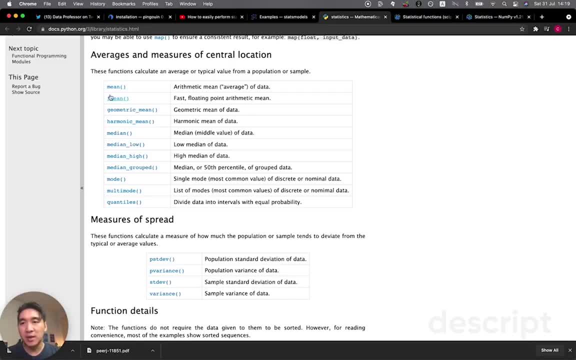 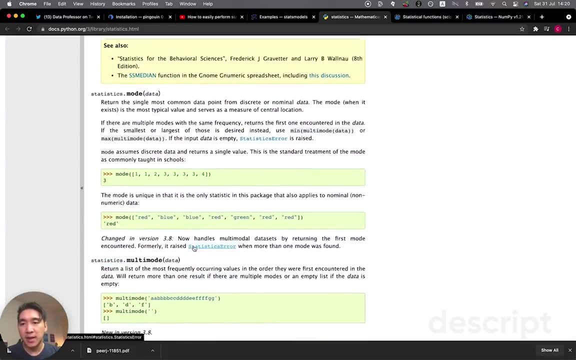 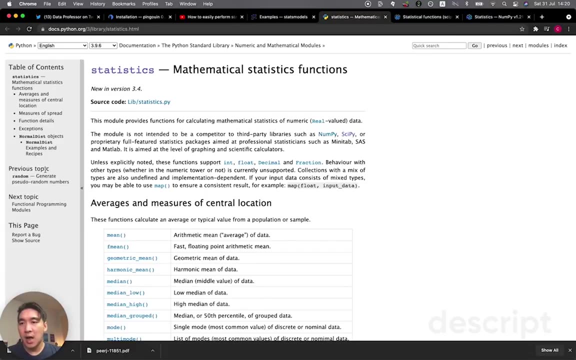 use, such as performing some basic quantiles, some basic arithmetic, mean median mode calculation. Okay, so these are the examples on how you could perform such analysis. More examples here? Okay, so, not feature packs, but it allows you to perform some basic statistical calculations. So no t tests. 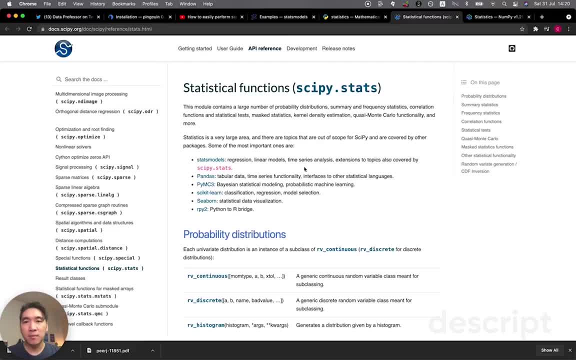 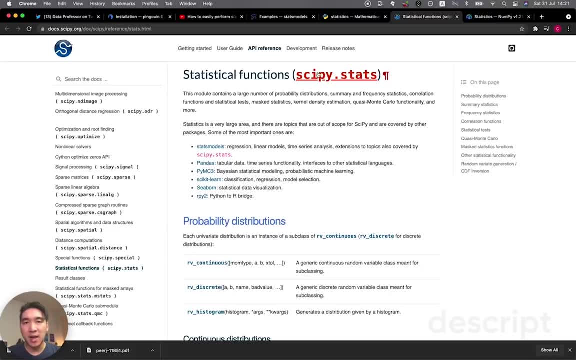 no ANOVA here, let's hop on to the next one, And so this one comes from the sci pi library. So let's have a look at some of the statistical functions that sci pi includes. So here you can see that it has some probability distributions functions, some basic summary and frequency. 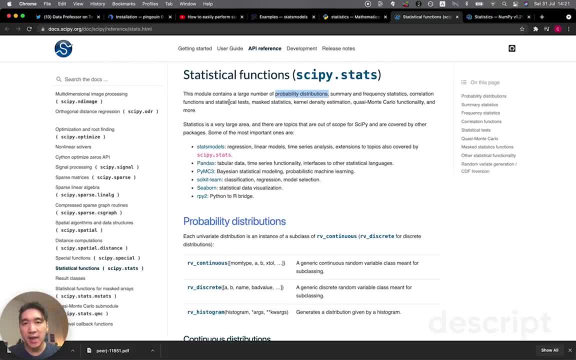 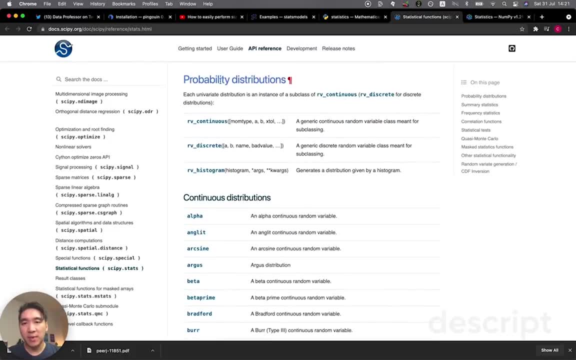 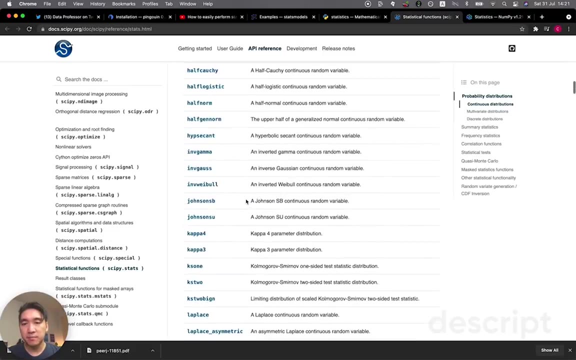 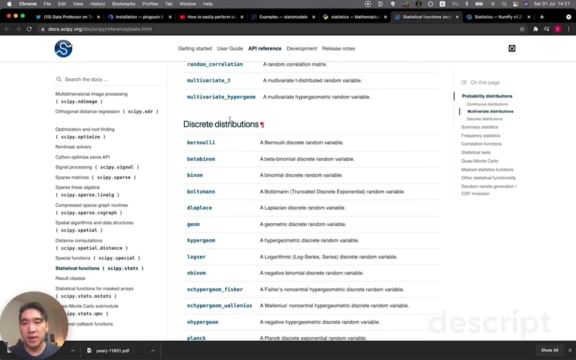 statistics, some correlation functions and statistical tests, as well as some kernel density estimation functionalities. Let's have a look at the probability distributions. So these are some of the functionalities here. These are for continuous distributions And you can see there is an exhaustive list here: multivariate distributions, discrete distributions. 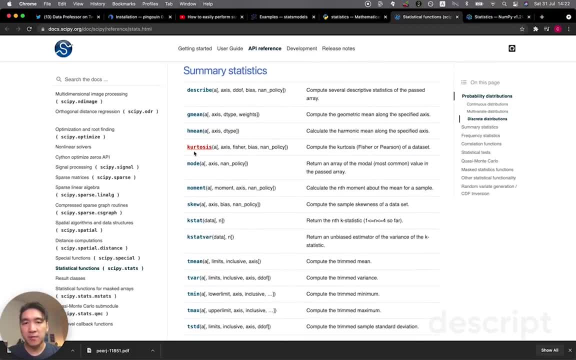 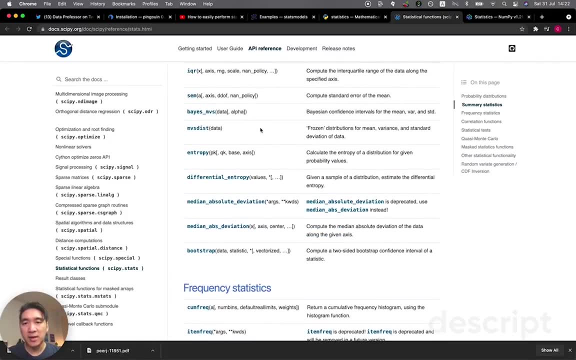 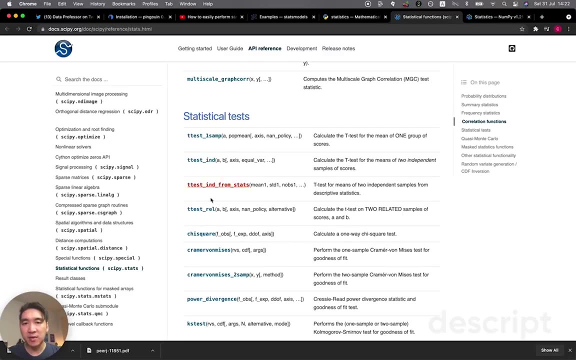 some basic summary statistics. you could even calculate the kurtosis. So this is more in depth than the one Provided by the Python standard library And you can see that the list is quite exhaustive. And you could also perform t tests as well here. critical wallace, So it has some. 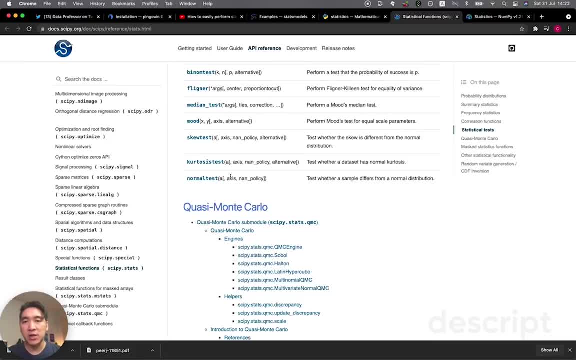 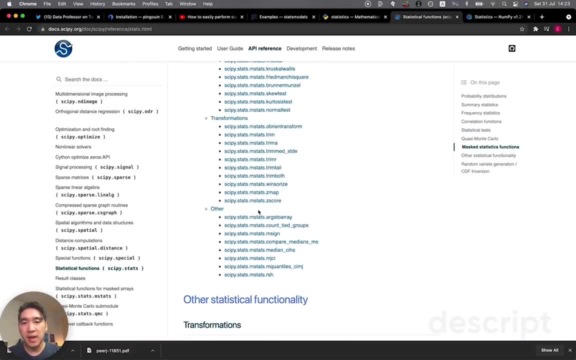 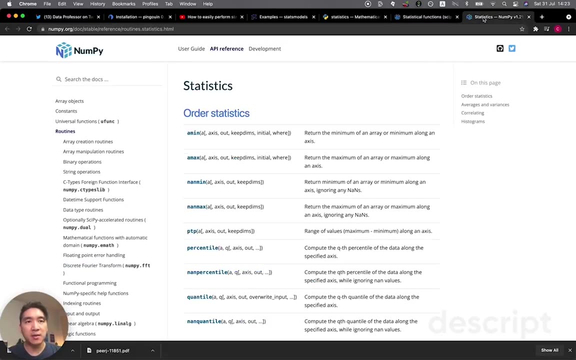 functionalities for performing parametrics and non parametric statistical analysis. These are some quasi Monte Carlo, So you can see that the list is pretty exhaustive. And let's hop over to the next one, And this is this. one is provided by NumPy, And you can see here that the number of functionalities 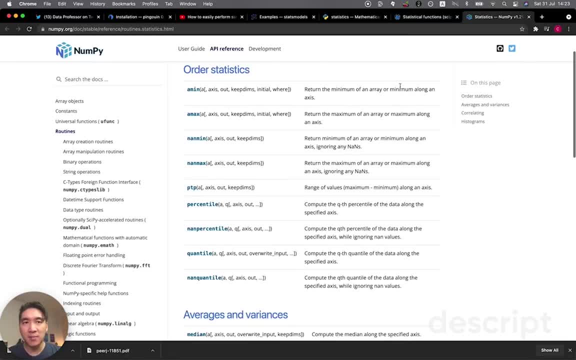 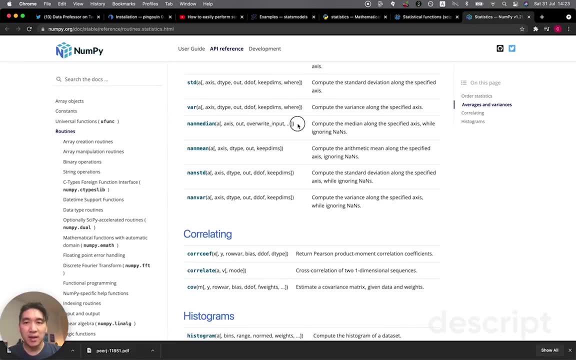 for performing statistical analysis is quite limited compared to the sci pi one. Some handy functionalities. here are the ones that allow you to calculate the median mean, standard deviation and also the variance, while at the same time ignoring the missing values. So this comes in handy when you have missing data in your data set. 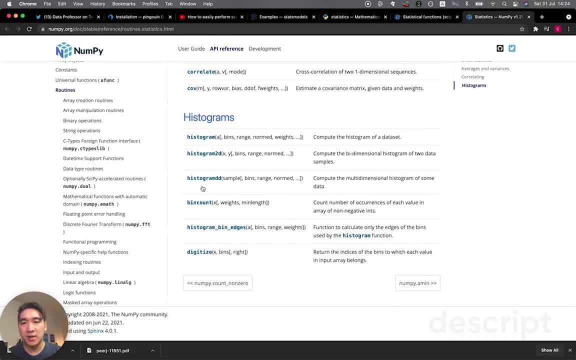 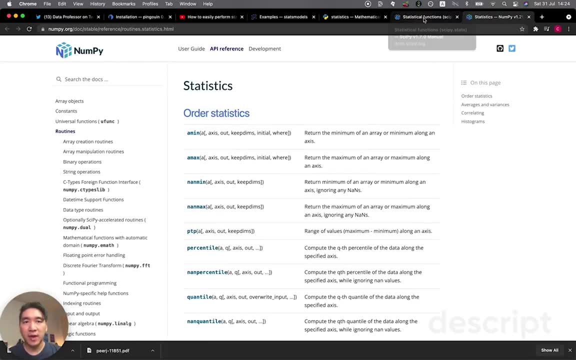 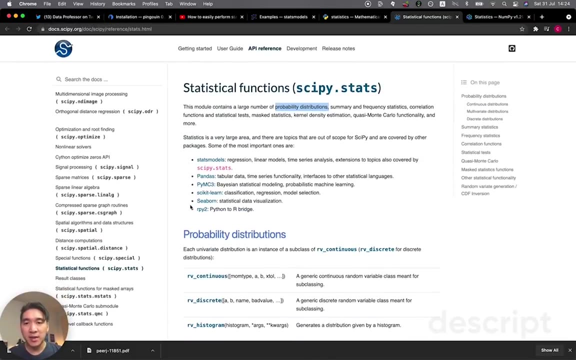 Okay, so some basic correlation functions. histograms: Okay, so not that feature rich, but still it might be useful as well. So, briefly, I saw some lists here that mentions about some other statistical libraries that I did not mention in the tweets, So let's have a look here. 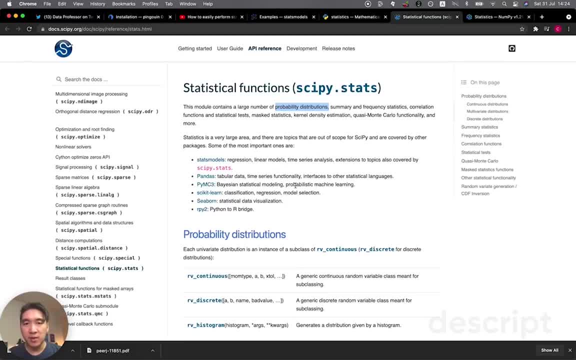 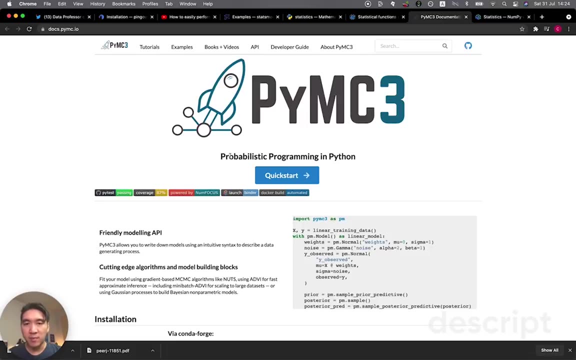 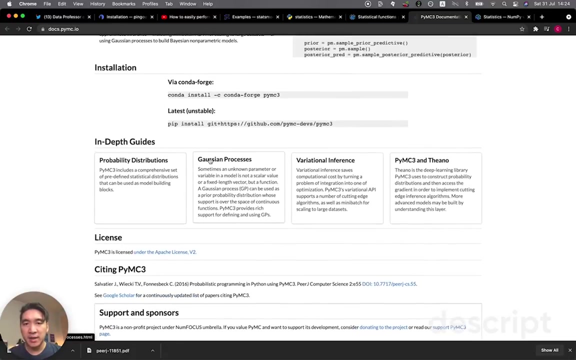 So there is this one, the Bayesian statistical modeling, and also probabilistic machine learning. Let's have a look here at pi MC three, So this one provides you the ability to perform probabilistic programming, and Python, So it has some probability distributions, Gaussian processes, variational inference, even publish. 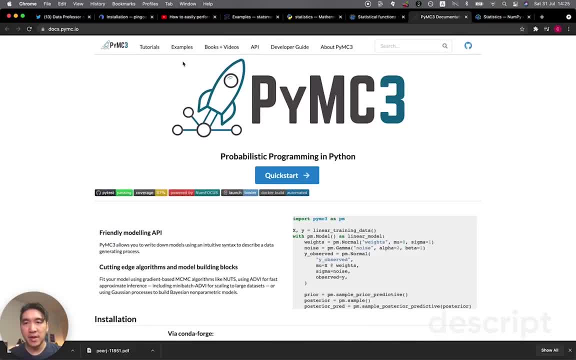 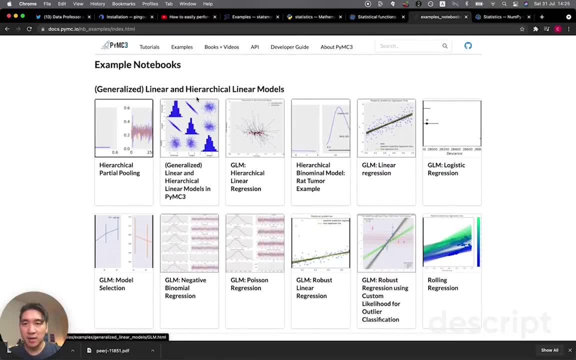 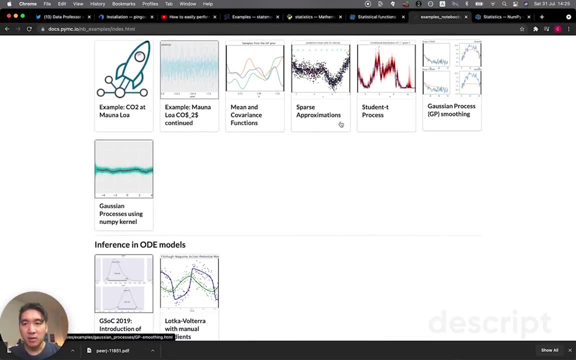 it in pure J computer science, Right, And so let's have a look at some of the examples here. All right, so my first impression here is that it's very nicely formatted, And so there are quite a lot of examples that you could follow along. 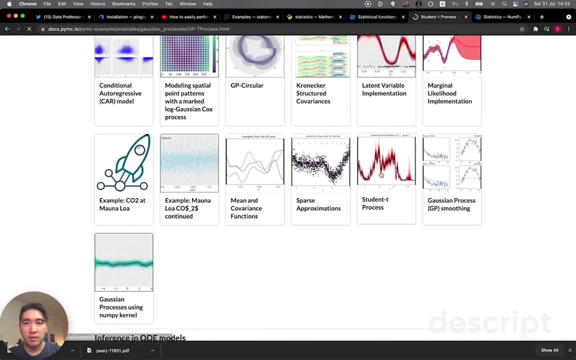 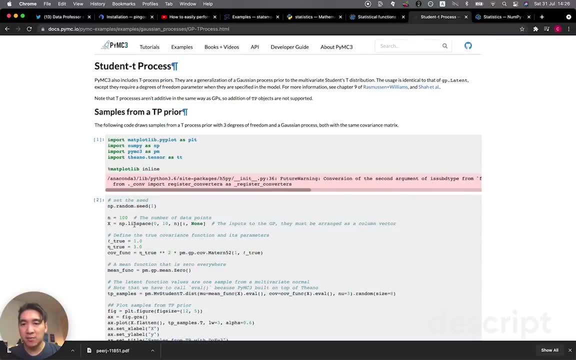 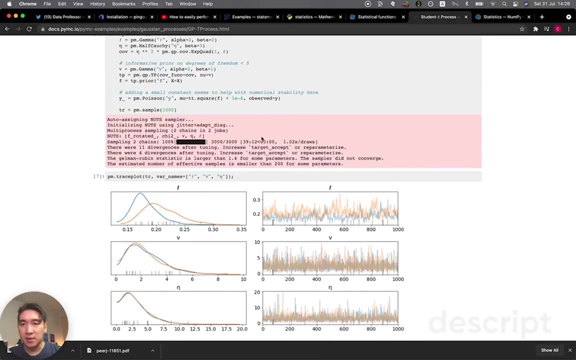 Let's have a look at here, So you could see that it's essentially a Jupyter notebook, And they provide you with some example data set that is randomly generated And then it allows them to create these plots And also some other analysis. 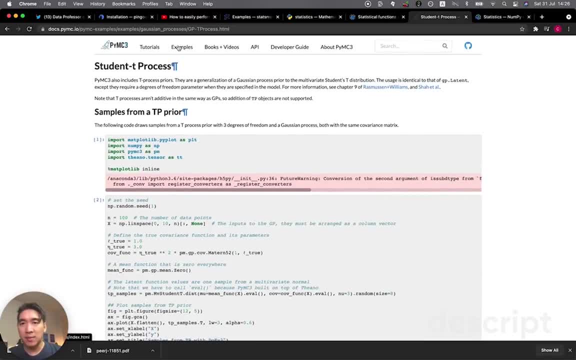 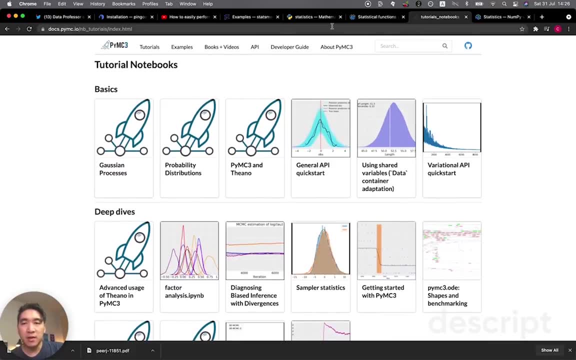 As demonstrated here, And so you could play around with some of the examples and tutorials as well, And so I'll provide you the link of this pi MC three as well in the video, in the video description, And let's have a look back at the tweet. There were a couple of 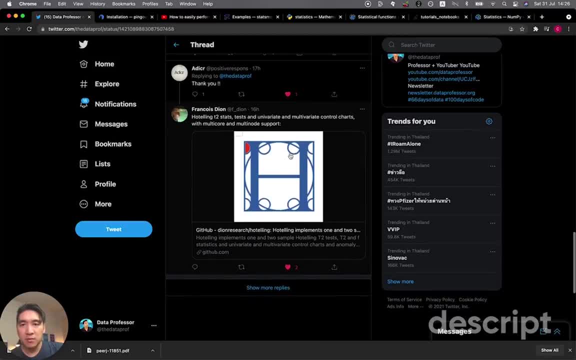 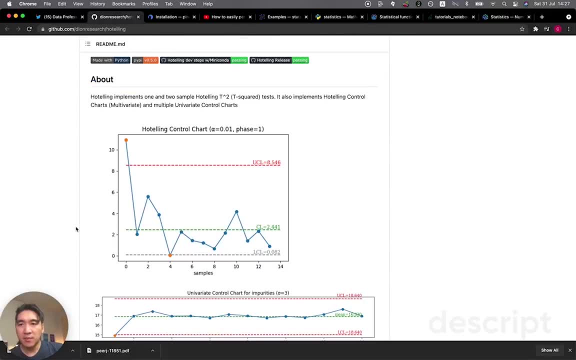 suggestions, Let's have a look. So Francois suggested this whole telling plot. Let's have a look at it. So in some of the research that I've previously implemented, one of our work we use Is the whole telling plot to examine the outliers in the predicted results, And so so this particular